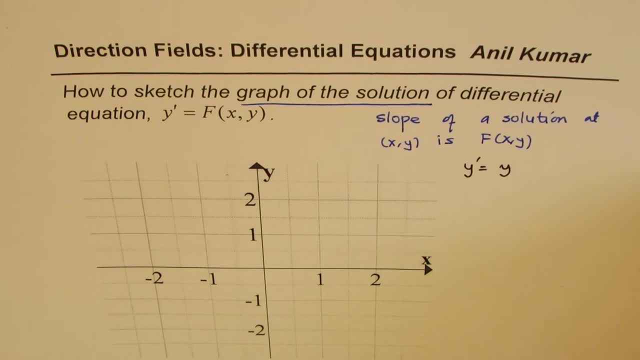 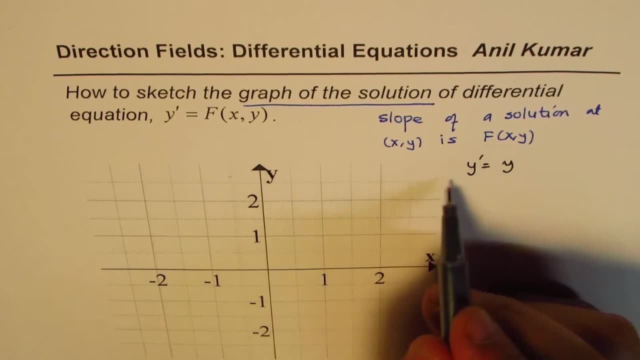 means that any point on this coordinate axis will have slope of y, representing the solution of this differential equation Right? We need not know what y is Right, But what we know here is that if y is 0, then y dash is 0. So So at this point, when y is 0, y dash means. 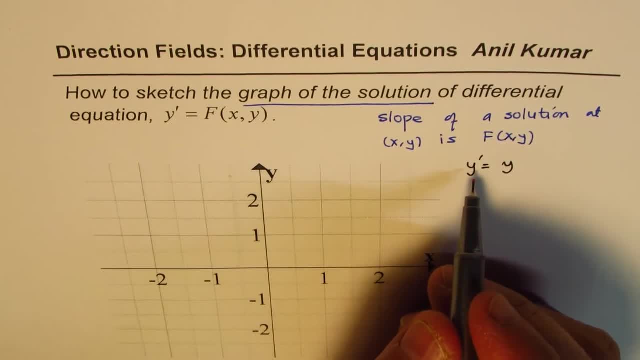 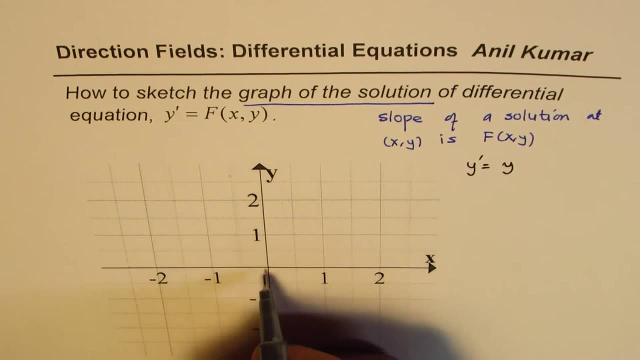 slope of the graph of the solution is 0.. Do you understand, Right? So at y equals to 0, the whole x is Right, And this x and y axis. So all along the x axis, y value is 0.. So this: 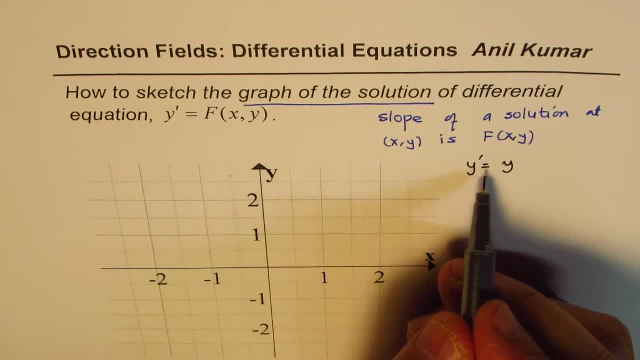 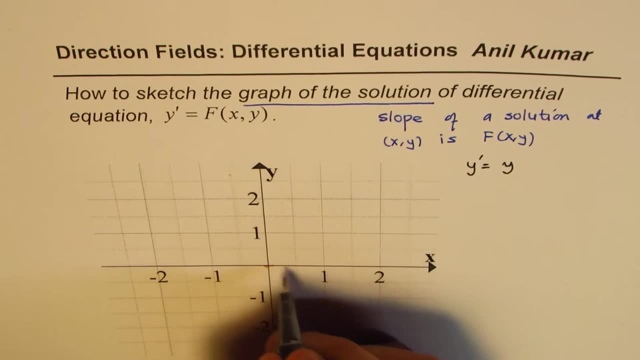 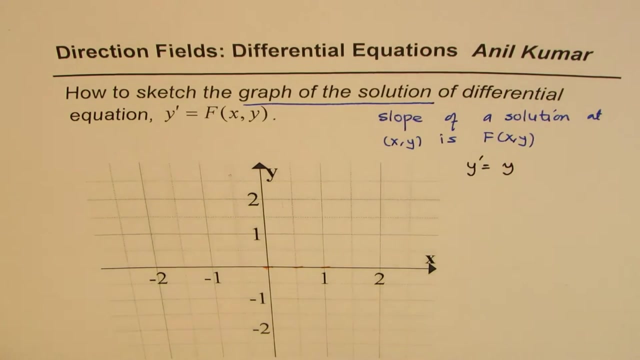 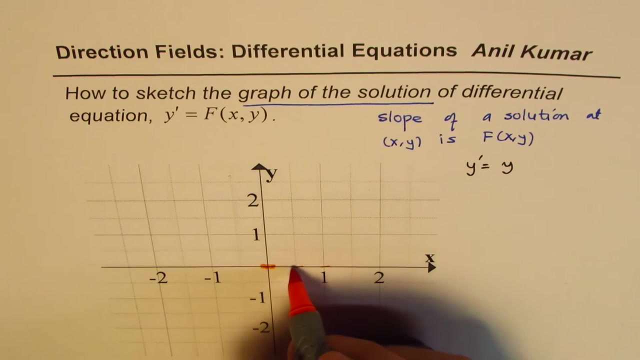 says that the derivative of the solution of this function is 0 all along the x axis, which is where y is 0. So we can draw short lines representing that solution. Let me use a highlighter pen so that becomes easier for us to see. OK, So the bold big one. So if y is 0, y dash. 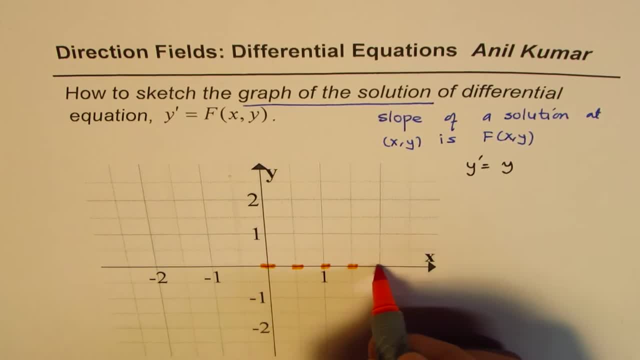 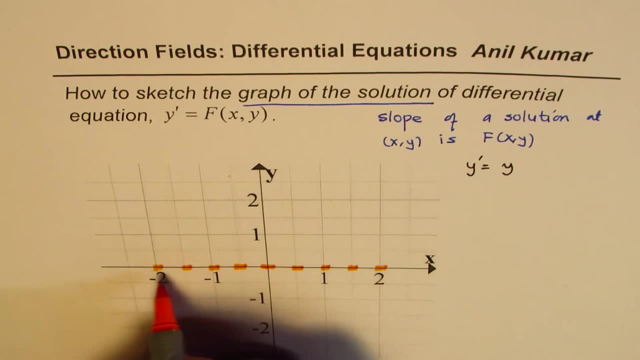 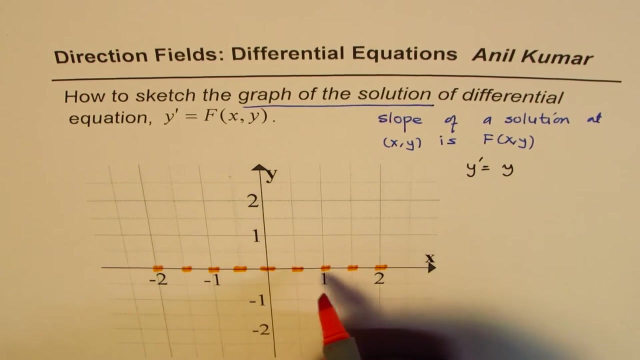 is 0. That means the 0. Right. So that means these small lines represent the slope Right From this differential equation. So all along the x axis Where y is 0, y prime is 0. So horizontal line represents that solution, Correct If? 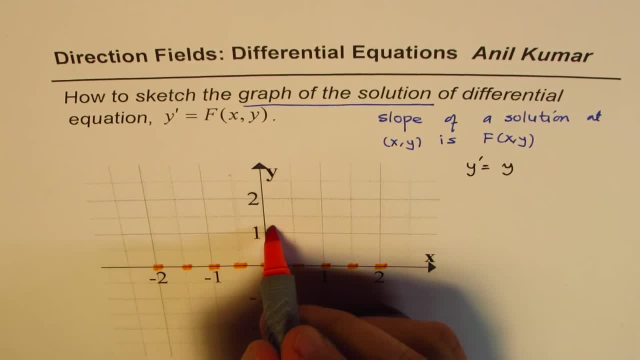 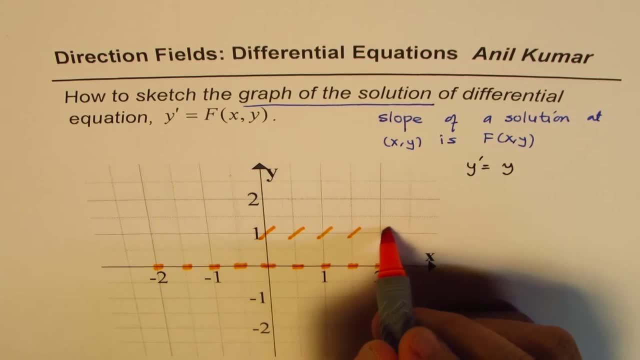 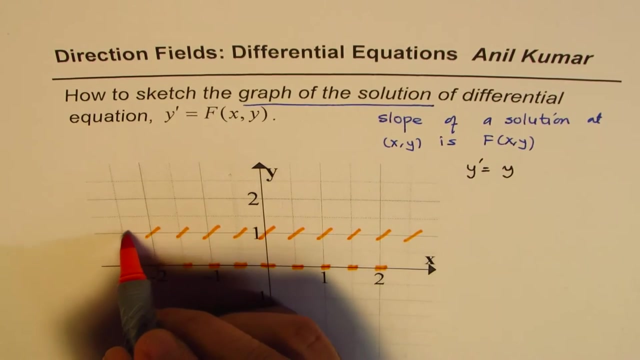 y is 1, then the slope is 1.. So I can draw a line like this representing the slope Right. So if I draw all along in the same direction, that shows that this solution curve will have this kind of a slope when it passes through this point, Correct? 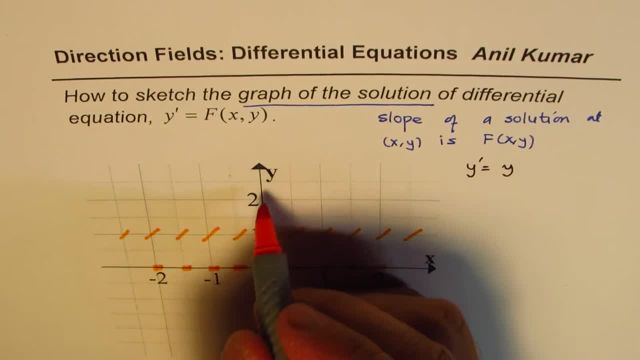 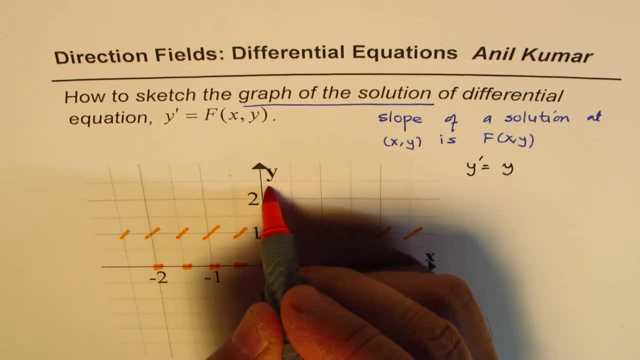 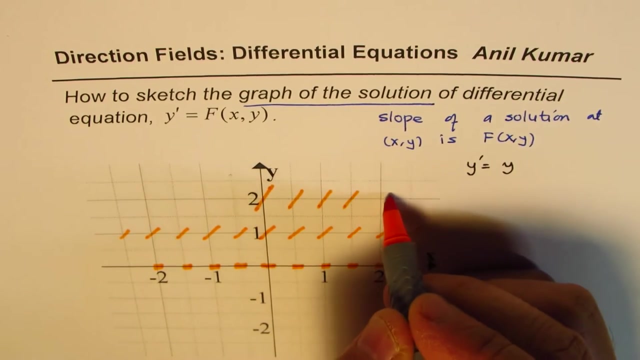 If y is 2, then then the solution will be: The slope will be 2 at that point. So all along this axis, y is 2. Right, Parallel to x axis. So let me draw the slope represented by these dashed lines. They only represent the slope at a specific coordinate point. 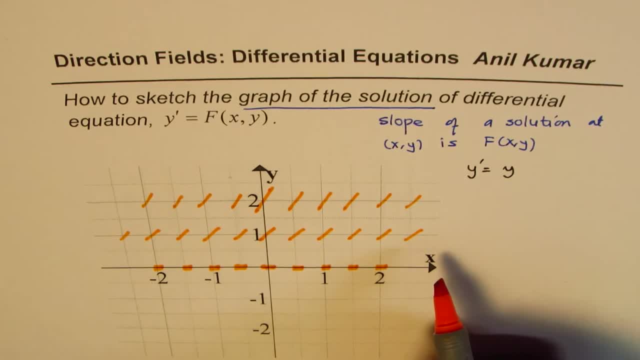 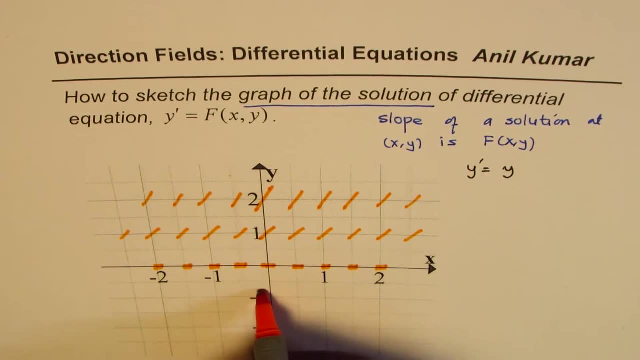 Right Which is given to us from the equation itself. If y dash is, let us say, negative 1. In that case, the slope will be negative 1. So it will be kind of like this: Do you see that? So if we do that, we can fill this up And at each and every coordinate point, will. 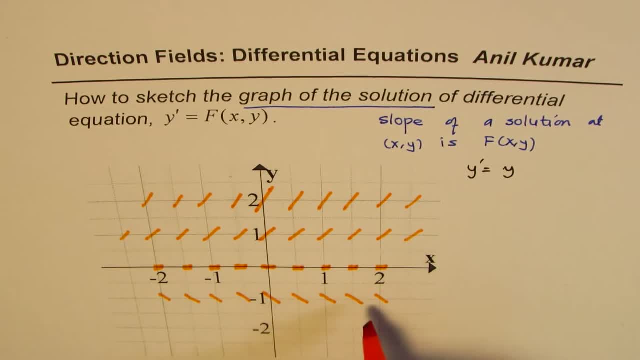 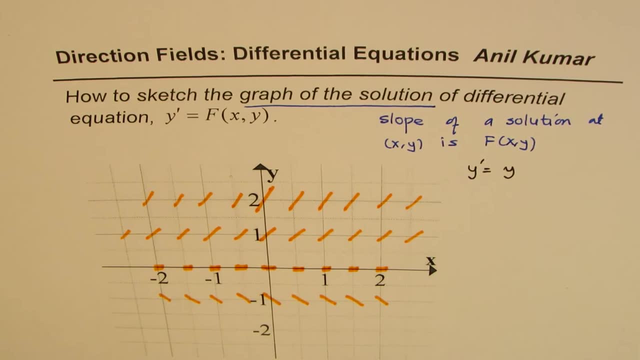 indicate the direction in which the solution curve moves Right Now let us assume that we also know from where the curve passes. There could be many curves which could move in a way, So that this direction thing is satisfied Right. But if we know that there is a point, 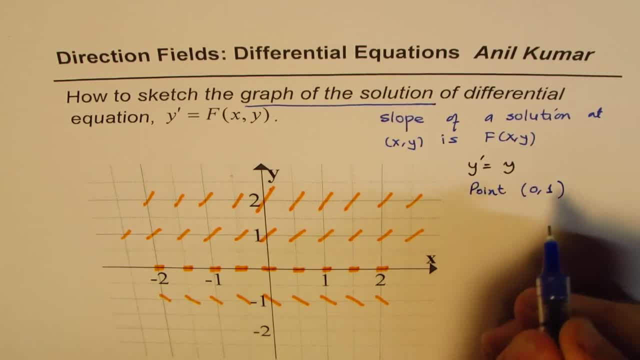 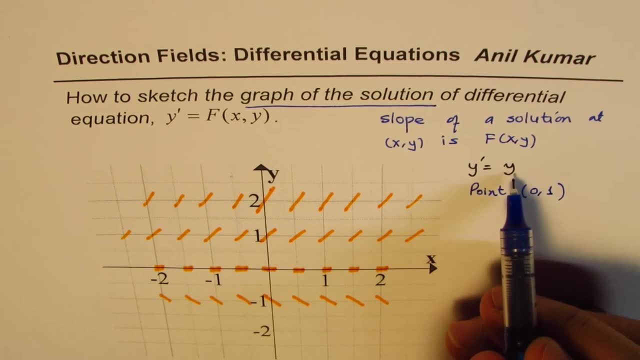 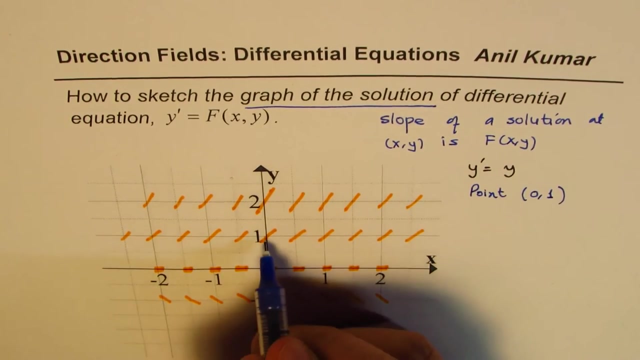 Let us take a point, Let us say 0, 1.. And we say this differential equation, y dash equals to y represents a curve which passes through the point 0, 1.. Right, So that means we know at least the starting point. 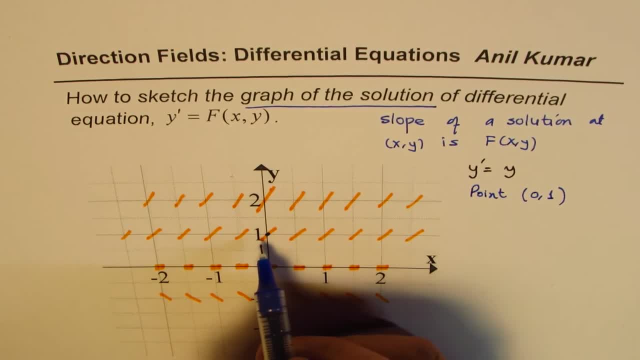 If we know, I should say That there is a point on the curve. So if we know a point and if we know in which direction to move, we can sketch the graph. You get an idea Right, So that's the point, we can start. 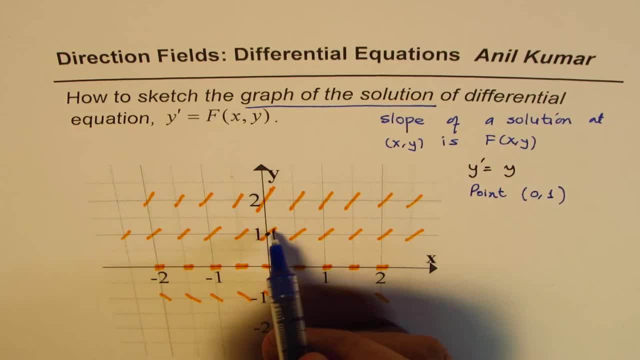 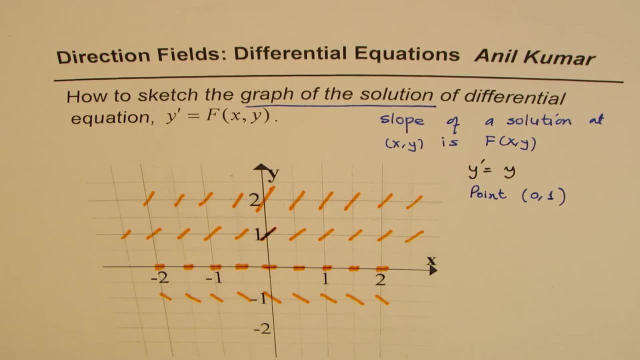 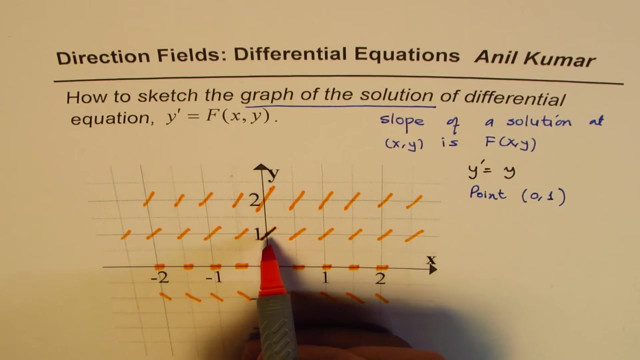 from and knowing that this is the direction in which we have to move, We know exactly how the solution of this differential equation can be represented as a graph. Now, if I take a points which are even closer Right, Then I can A fairly accurate graph. So if y is, let's say, 0.5, then y dash will be 0.5.. So let me 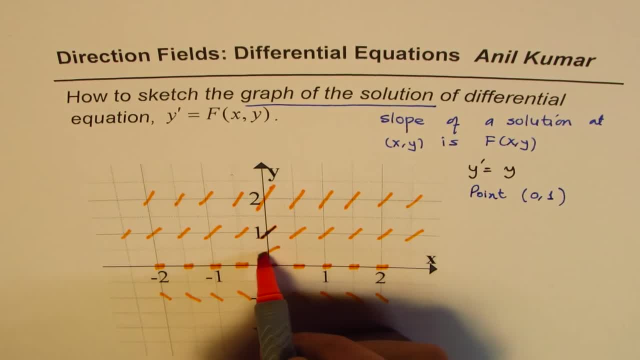 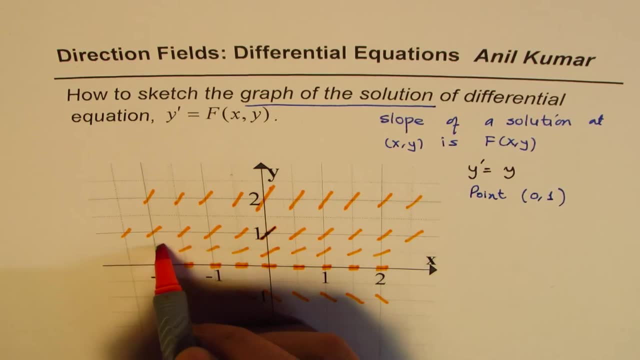 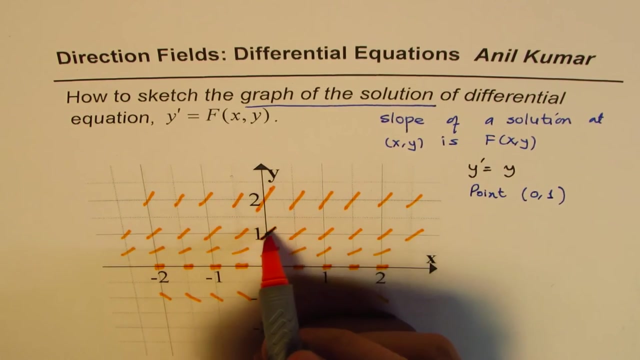 represent this line with slope of half Right. So let's say these are the small dash lines representing slope of half all along this line, Right. Similarly, if I have a point y, coordinate point, as 1.5, then the slope would be represented more than this, less than that. 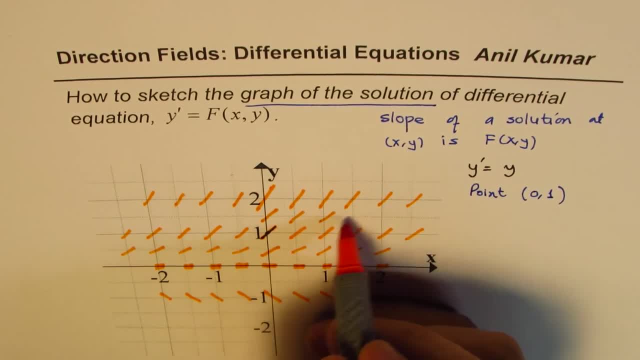 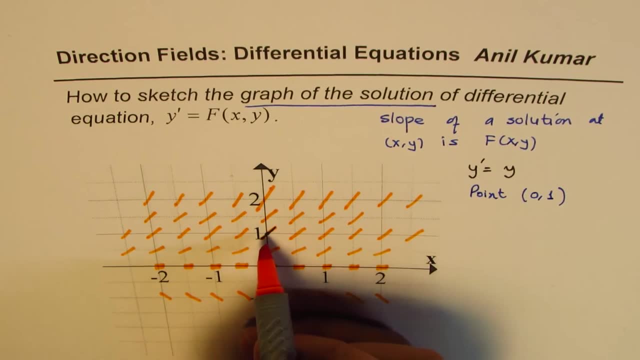 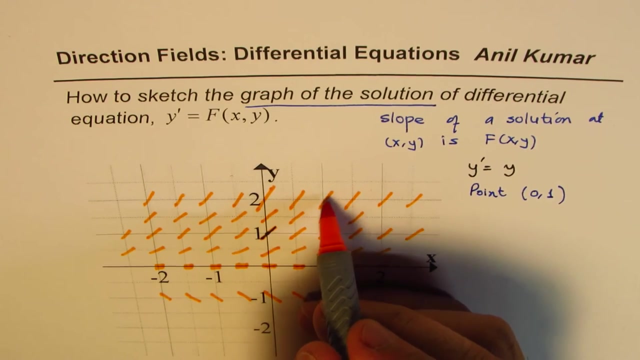 So kind of like this, Right, You see that So. so all these points represent that kind of a slope, Right? So, knowing all this, we can easily actually sketch the graph, Right. So here, if it is 2.5, the slope will be steeper than this. So it could be kind of like this: 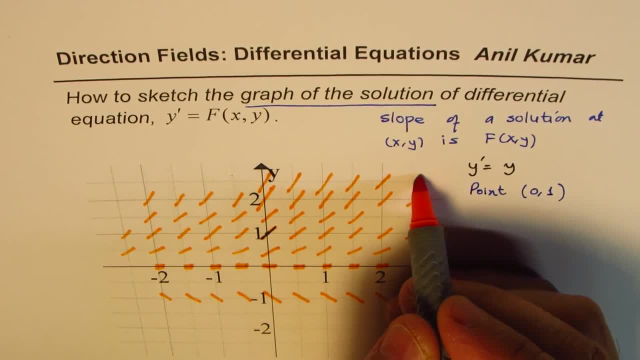 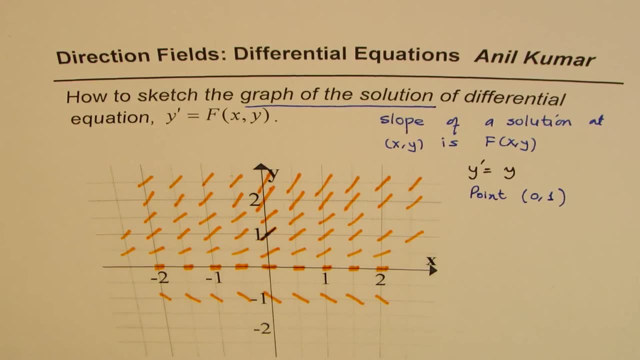 Do you see that? So we can sketch these dashed lines, which represents the slope of the solution. Now, once you sketch this, you see a pattern, and this pattern is called the direction field. It represents the direction in which the solution of the differential equation curve moves. 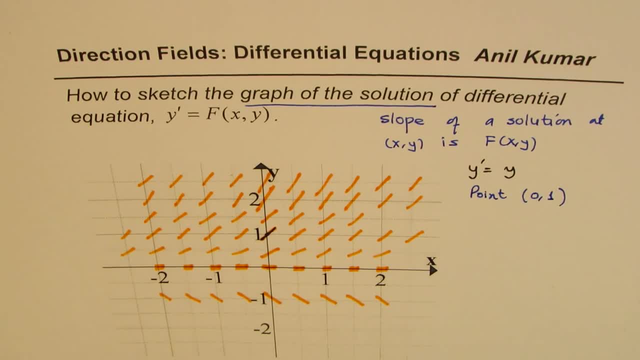 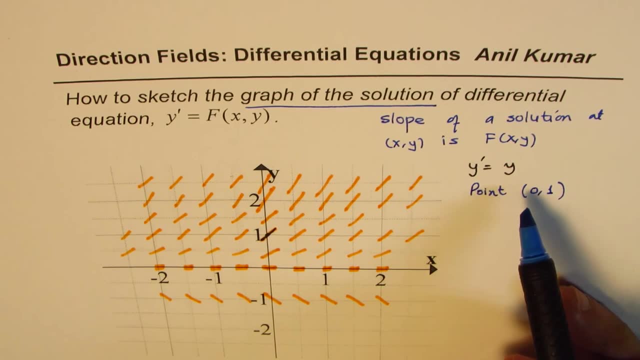 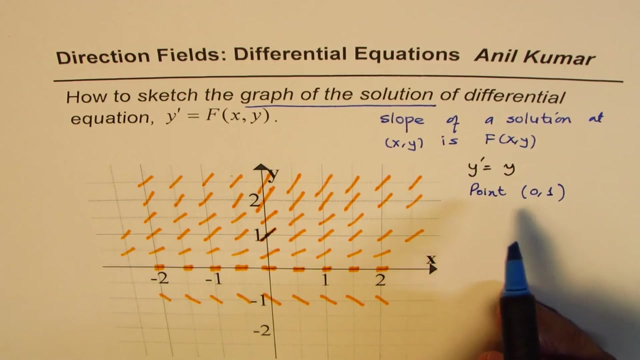 You get an idea. So that is how we can utilize direction fields to find solution of differential equation, even without solving them. So if we know a point, we specifically know which curve We are talking about Right Now, since we know that the point is 0, 1, through which the 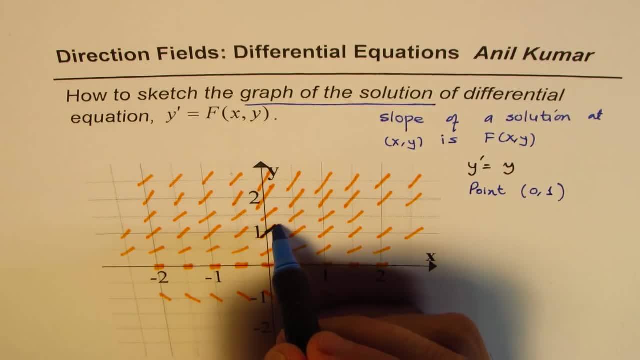 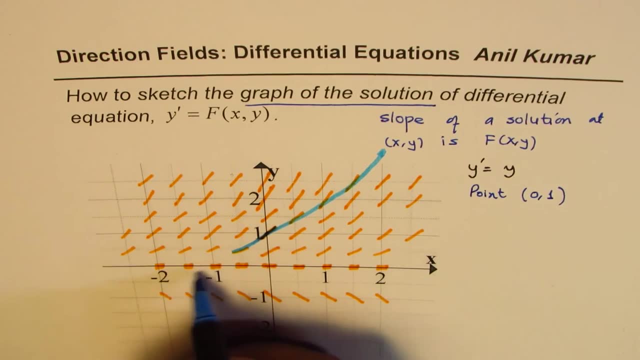 curve passes. we can start from here and then move along the direction, as they are saying. Do you see this? These lines are indicating the direction and you know, as you go it is horizontal approaching. We could have a curve Right, So we do get a curve, which is looking. 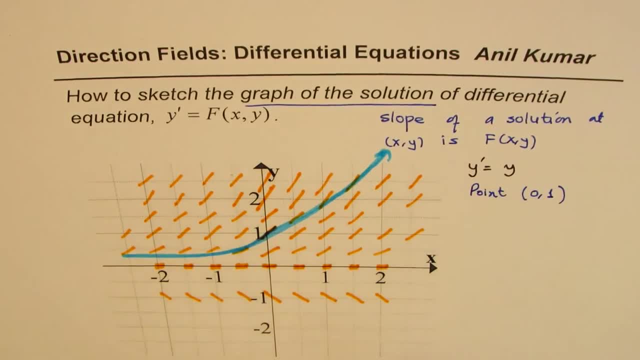 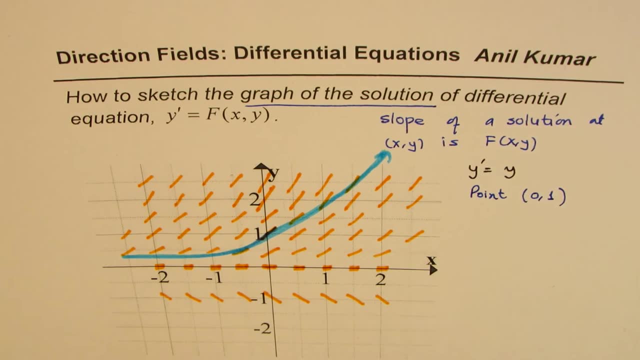 like an exponential function. Do you see that? And that is what the solution of this equation is. So These directions of the field give us an idea of how to sketch solution of a differential equation without explicitly finding its solution. This is a very, very important concept. especially, you can use it for collecting data from the 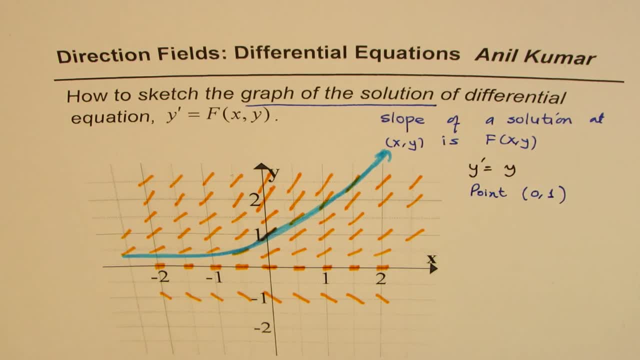 experiments. Now, when you collect data from experiments, it may be very difficult to get some equation for that data Immediately, but sketching a graph gives you an idea of the type of solution you might be expecting. I'm Adil Kumar and I hope you appreciate this concept. you can always. 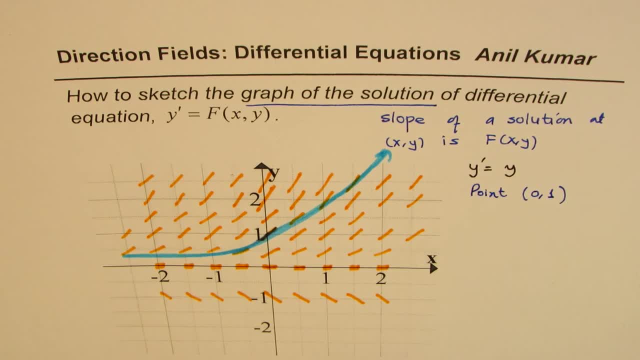 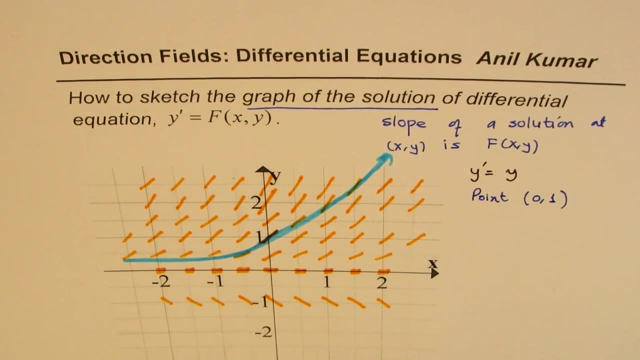 share and subscribe to my videos like, if you like, and I'll add few more to explain and practice direction fields and how to graph solution of differential equations using them. thank you and all the best you.